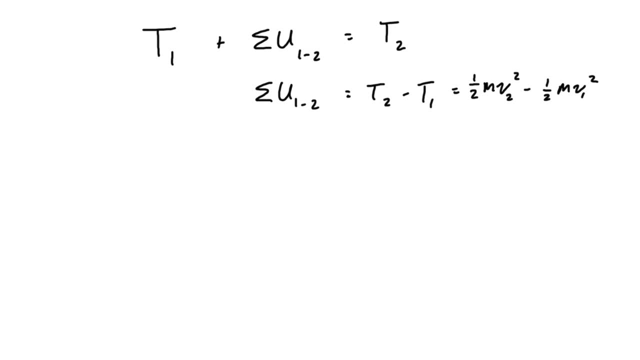 set up a problem here, where we're going to find friction and we're going to find the work done on this box that's sliding across the floor with an initial velocity that comes to a stop after a distance of 1.5 meters. So let's just change the color so we can see what we're working. 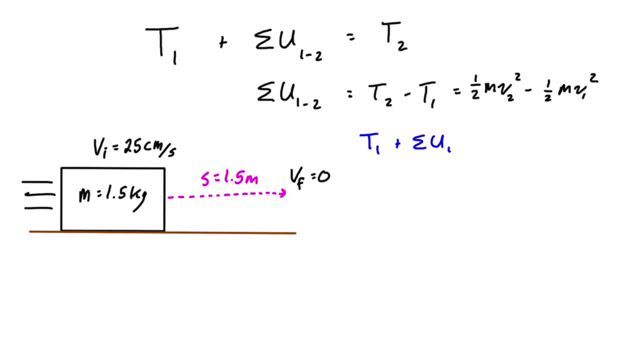 with and we have T1 plus the work done is equal to T2.. So let's expand this out a little bit. We have 1 half mv1 squared for the kinetic energy plus the work done. That's just going to be the force of friction. 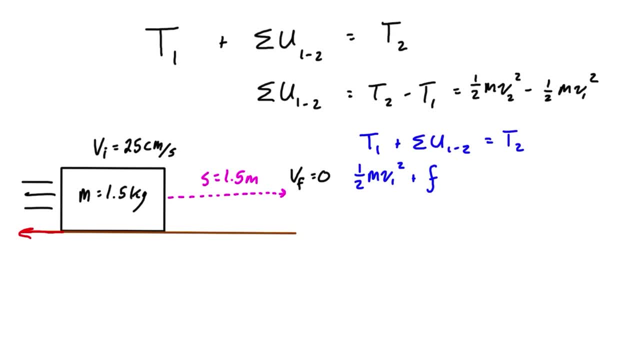 So we'll label that. on going this way, going the opposite direction to the distance being traveled, And that's going to be times cos theta s where theta is the angle between the direction that we're going, the displacement and the component of the force that's in line. 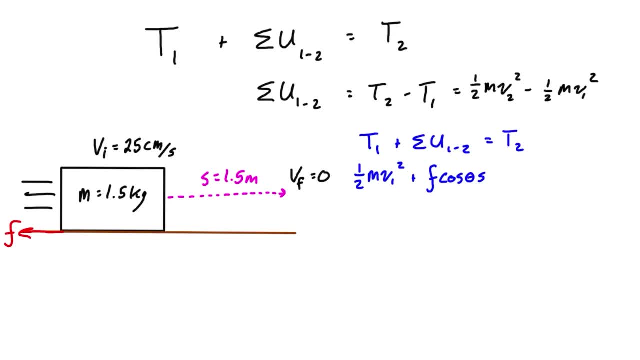 with that. So in this case it's going to be 180 degrees, because it's opposite, And this is all equal to kinetic energy at the end, and that's going to be 0, because the final velocity is 0.. So if we bring the 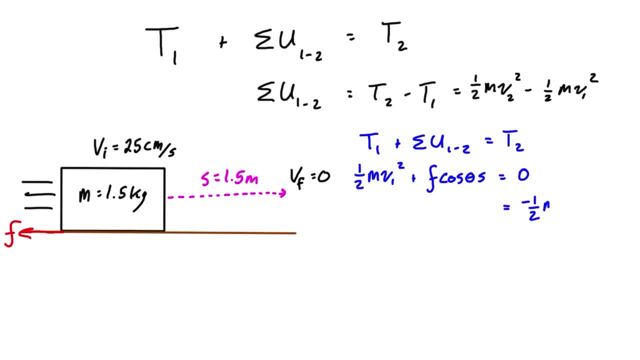 1 half mv squared to the other side, it's negative 1 half mv squared. And f times cos of theta, well, cos of 180 is equal to negative 1, that's times s. So we can then get rid of the negative on both sides and we can bring the s down to the other side. So we're 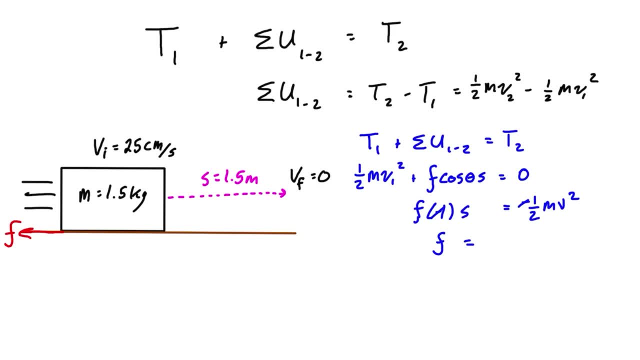 left with the force of friction is equal to mv1 squared over 2s. We're going to run out of room down there If we just bring it over to the left side here. So the mass is 1.5 kilograms times the velocity, which is 0.25 meters per second. 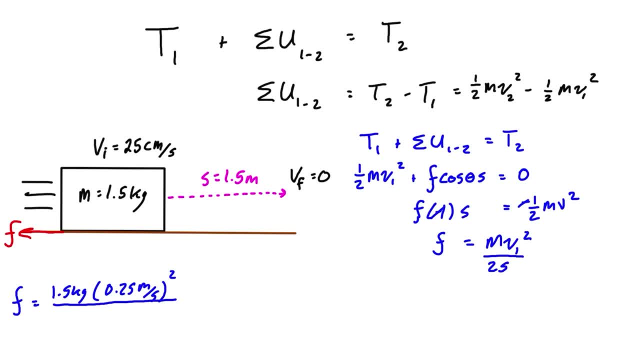 It has to be in meters per second And that's all squared, And this is over 2 times 1.5 meters for s. So that's going to give us friction force of 0.03125 R p c 0. So this